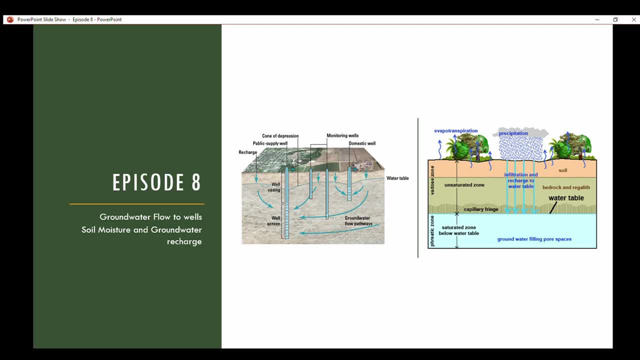 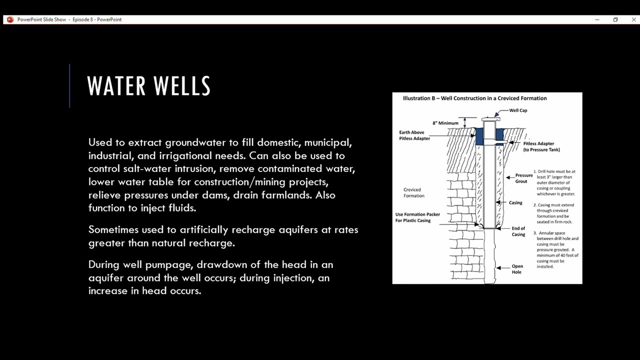 eight will be covering two different chapters: groundwater flow to wells and then soil moisture and groundwater recharge, And so a water well. it's used to extract groundwater to fill domestic, municipal, industrial and irrigational needs. It can also be used to 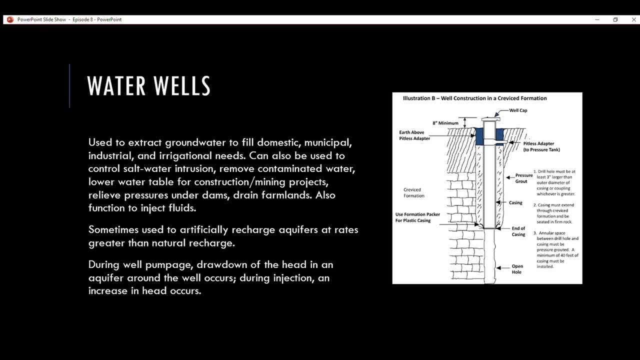 control saltwater intrusions which occur off of coastlines. Ocean water contaminates aquifers, freshwater aquifers. It removes contaminated water, which is what I dominantly do. It lowers water table for construction or mining projects. It relieves pressure under. 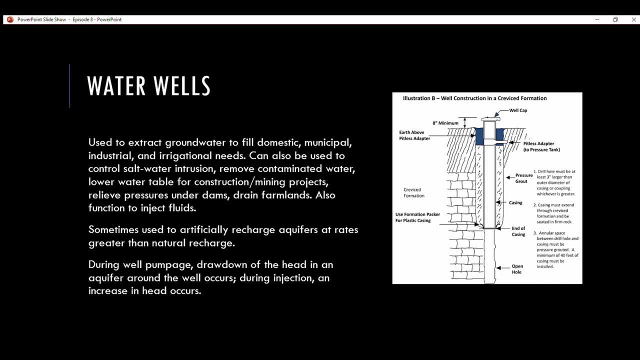 dams and it drains farmlands. Also, you can use water wells to inject fluids into the aquifer. Sometimes it's used to artificially recharge aquifers at rates greater than natural recharge, and that would typically happen in, say, an arid region. 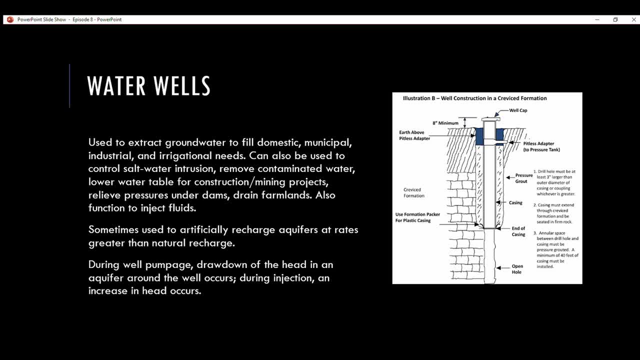 So the water table is probably falling during summer. so you want to add some of the water from the nearby river, for example, to kind of raise the water table. So during well pumpage, the drawdown of the head in an aquifer around the well occurs During an injection. 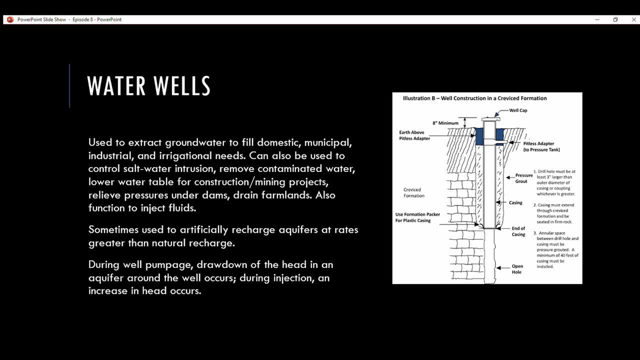 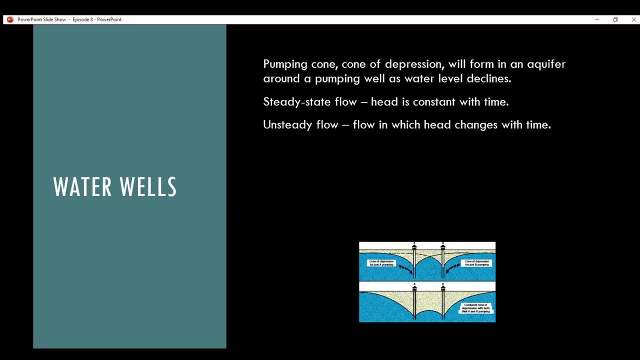 the increase in head occurs. Slide 8. So the pumping cone or conodipole. Conodepression is what forms when an aquifer around a pumping well is pumped And as the water level declines it'll form this cone. It's called a conodepression. 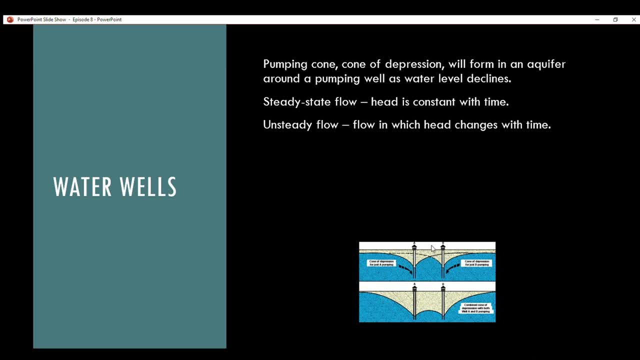 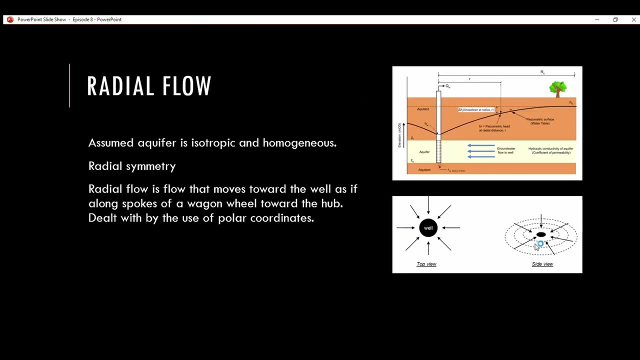 And steady-state flow is when head is constant with time and unsteady flow is when head changes with time. Slide 9- Radial flow- Slide 10. So when you're dealing with conodepression forms, when you're dealing with radial flow, 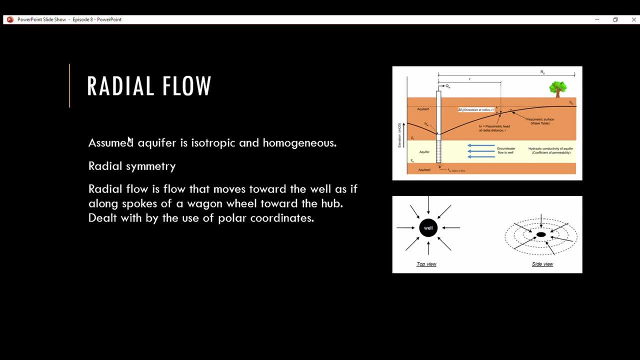 you're assuming that the aquifer is isotropic and homogenous. It has radiosymmetry And radial flow is flow that moves towards the well pictured over here, as if along spokes of a wagon wheel towards the hub. It's dealt with by using polar coordinates. 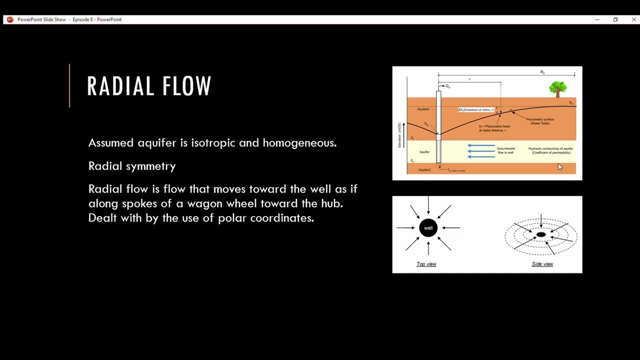 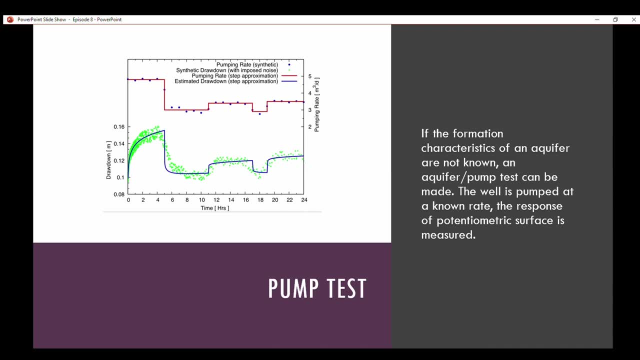 Slide 11. Slide 12. Slide 13. Slide 14, Slide 15, Slide 16, Slide 17, Slide 18, Slide 19, Slide 19, Slide 20. Scroll to the bottom of the slide and hit the button. Slide 19, Slide 22. 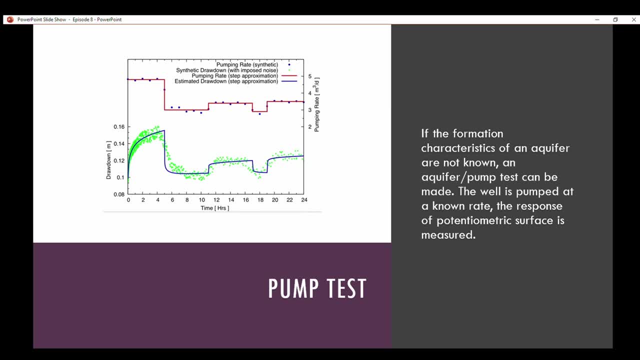 Slide 24, Slide 25, Slide 26, Slide 26, Slide 27, Slide 28, Slide 29, Slide 31, Slide 31, Slide 33, Slide 35, Slide 37, Slide专, Slide 44, Slide 49, Slide 51, Slide 53. you know, over five hours it'll reach. 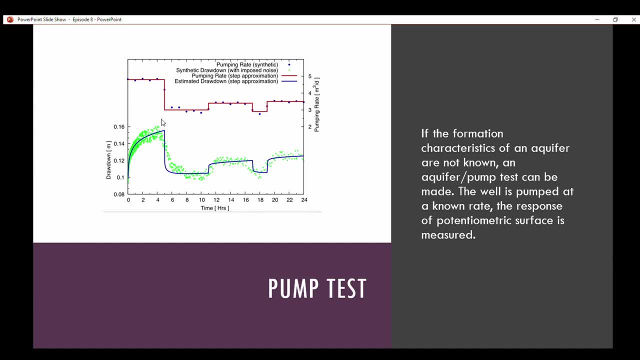 a what's it called steady-state on during this pump test. reach steady-state here and then significantly decrease and in drawdown and then you know you get a smaller one over here were steady-state isn't achieved anymore and starting creasing and those reach steady-state again. 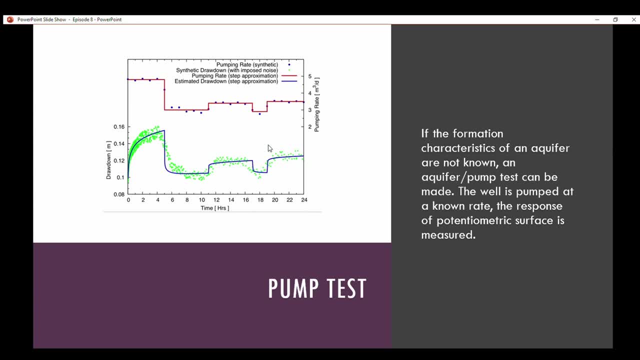 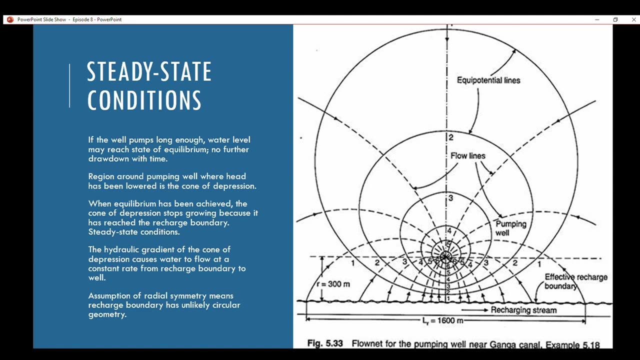 on. this gives you an idea of how well the the aquifer is transmitting water through it. so hydraulic conductivity, so steady-state conditions at the well. pumps long enough, the water level may reach a state of equilibrium, so no further drawdown with time. the region around a pumping well where head has been lowered is the. 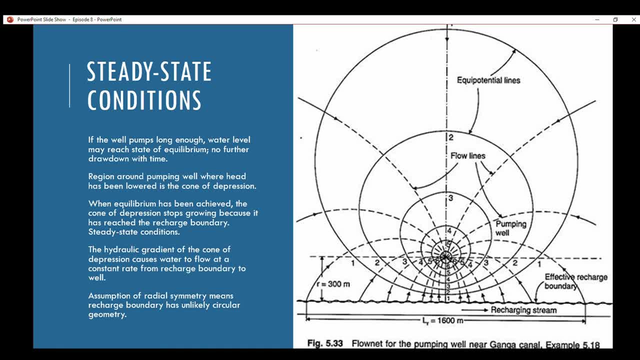 Kona depression. when equilibrium has been achieved, the Kona depression stops growing because it has reached the recharge boundary. which recharge boundary such a on this picture would be like it's a stream, for example, and that that would be steady-state conditions? the hydraulic gradient of the 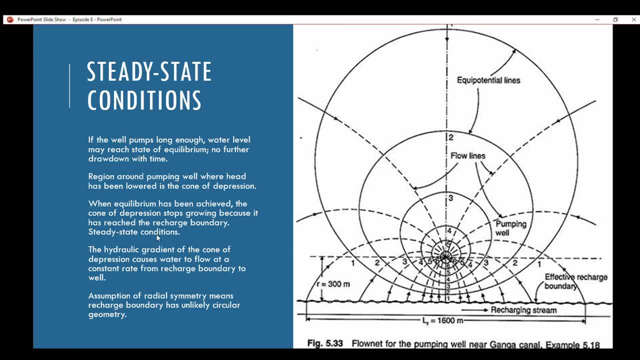 Kona. depression causes water to flow at a constant rain rates from the recharge boundary to the well, and the assumption love radio symmetry means that the recharge bound boundary has unlikely circular geometry. okay, so this one was in the book, but I think it's kind of important to 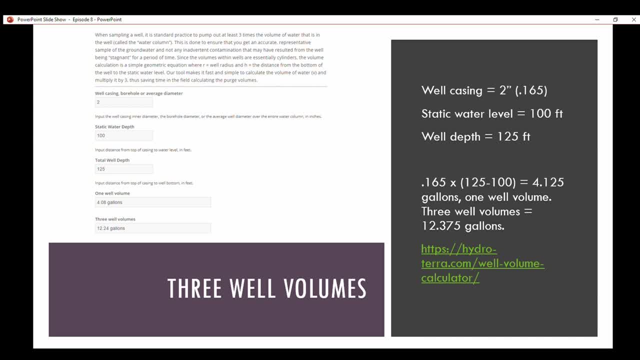 to to note. so when, when you're sampling a groundwater well, you typical role- at least where I work in the state I work in- is you wanna pump the well to three well volumes to get a representative for sample of the aquifer, because they believe that if it's just one well volume, that 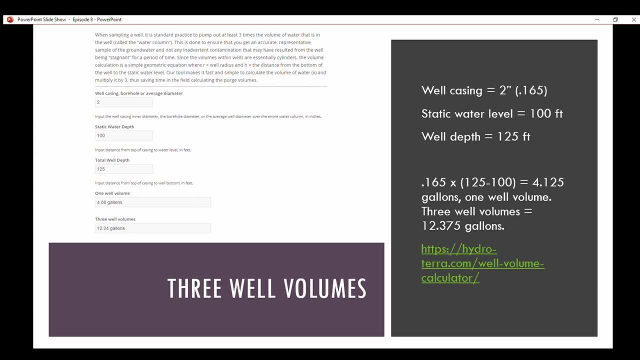 you sample from, the water has stagnated a little bit. so if you pump three, you're not getting that stagnated water, you're getting water that's coming from you know, and all around the well and in the surrounding areas its it's trying to reach equilibrium saw. 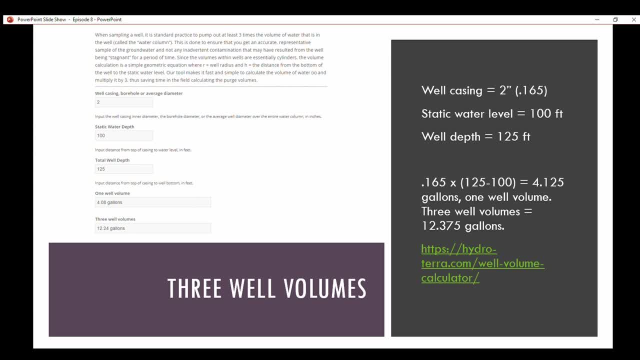 obviously more waters coming in through the formation and into the to what. where the well is, see, you can pump it out. um, so my calculation is pretty simple. you, uh, so say we have the well depth of a hundred twenty five and the static water level, or? 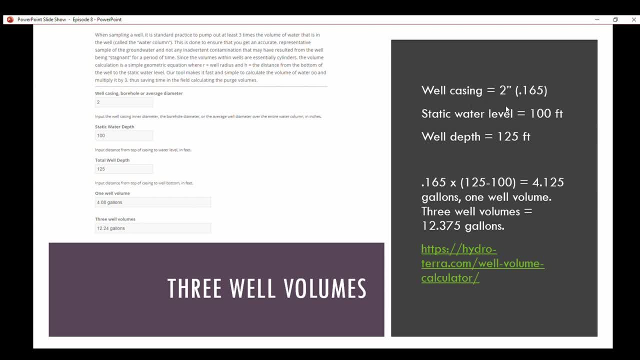 groundwater elevation level of one hundred feet. you subtract those to them and then multiply it, because the settling is two inches, that's uh, point one six five. so you multiply the difference between the static water level and well depth, the well casing, and that'll give you onewell volume which is 100 feet and twelve inches. so just put the level down. the right decision margin, pump character, divided up to 2 in, that's 2.165. so you multiply the difference between the static water level and well depth, and umthe well casing, and that'll give you one well volume which is just .165, and 3 in. 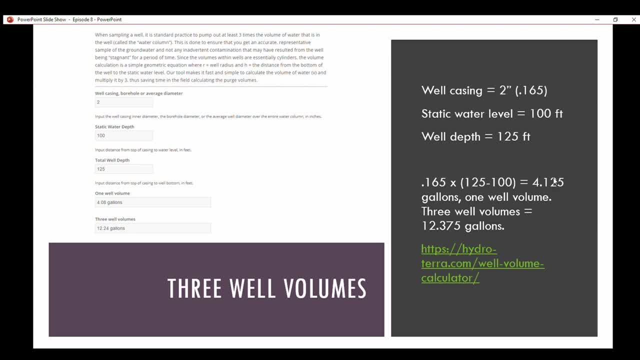 is in this case four point one, two, five, and you multiply that by three and you get twelve point, basically four gallons. after you've pumped twelve point four gallons out of this, well, that's a representative sample, potential sample. so that's when you would do your sample. okay, so a slug test. 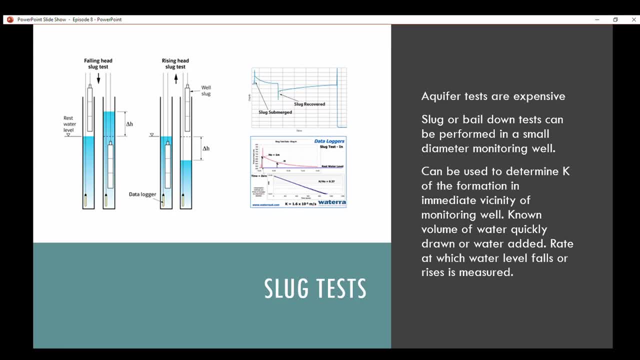 aquifer tests are expensive, so in this case you could use a slug or bell down test in a small diameter monitoring well. it can be used to determine the hydraulic conductivity of the formation in the immediate vicinity of the monitoring well. the known volume of the water quickly drawn or water added, the rate at which water level falls or rises is measured, and then 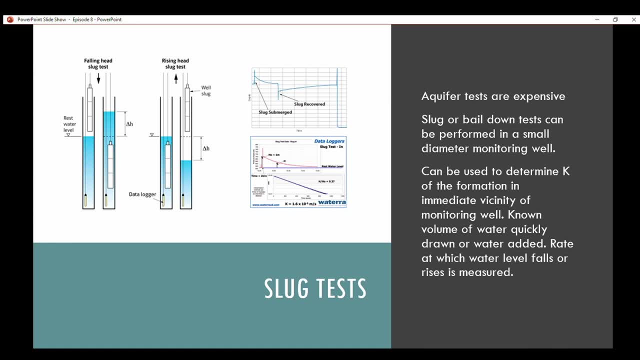 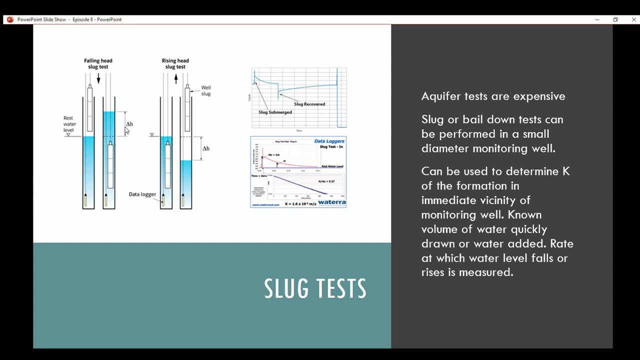 in height there, or you can measure the change in height in a rising head slug test and you know, over a certain amount of time as that, that change in head occurs. that can give you an idea of what the hydraulic conductivity in the, in the formation that you're taking the water out of, can be. 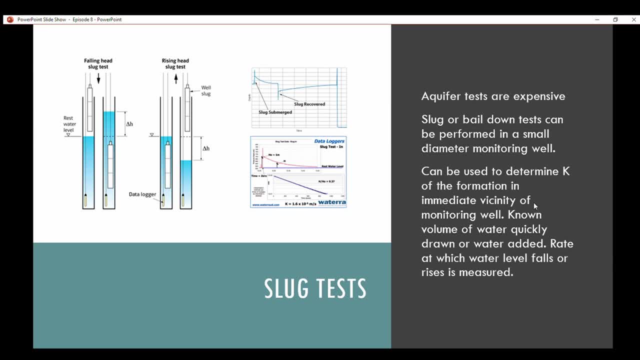 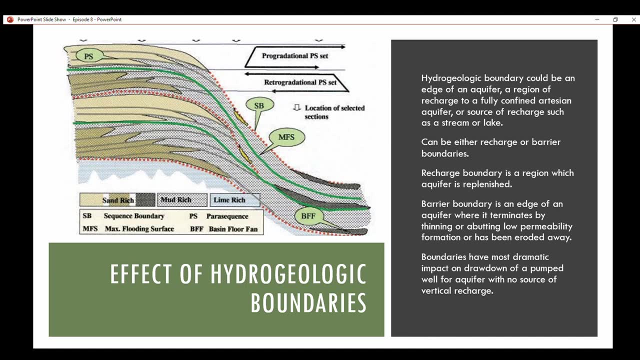 determined so the effect of hydro hydrogeologic boundaries. a hydrogeologic boundary could be the edge of an aquifer, a recharge, a region of recharge to a fully confined artesian aquifer or a source of recharge such as a streamer like it can be either a recharge or barrier boundary. a 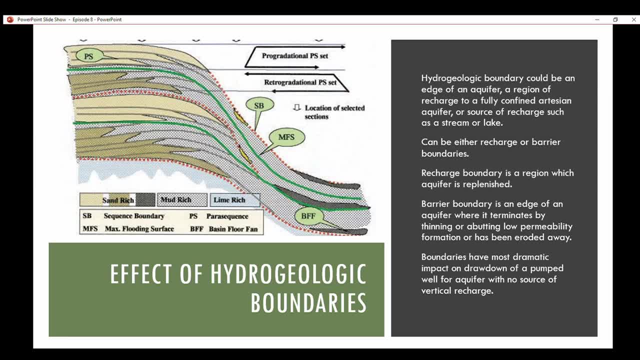 recharge boundary is a region where the aquifer is replenished, such as a stream or a lake, and then a barrier boundary is an edge of an aquifer where it terminates. by then, a barrier boundary is an edge of an aquifer where it terminates by thinning or abutting, low permeability formation or has been eroded way, which is why I included. 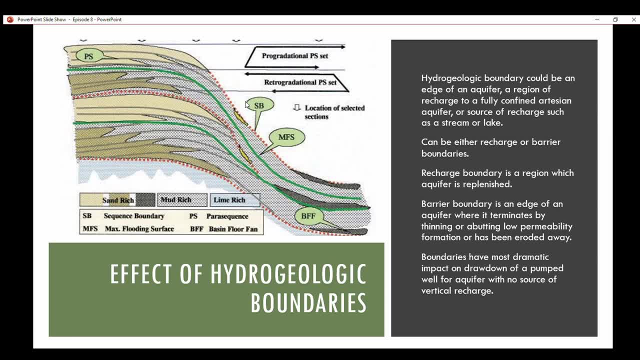 this picture. this is stratigraphy, if you guys remember this. um, it's typically looked at when you're dealing with petroleum geology, but this gives you an idea of the thinning and abutting. so this, this, uh, say this, what is this? a sandstone? the sandstone right here is a budding against a. 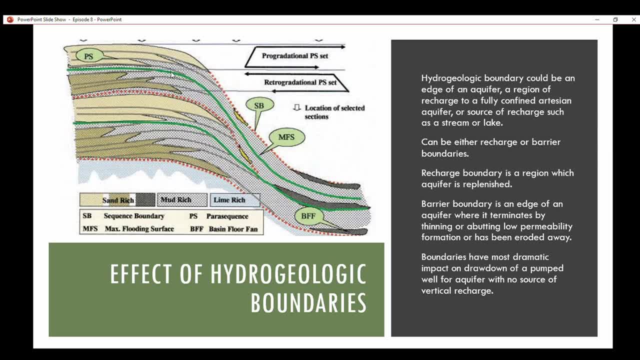 mud-rich uh formation. so obviously, the mud rich form is a sandstone in the form of a reinforced salvage, in the form of a reinforced salvage. in the form of a reinforced salvage, this is a gold leaf and you that would be an aquitard in this case, not a hydraulic conductivity, so this would be a 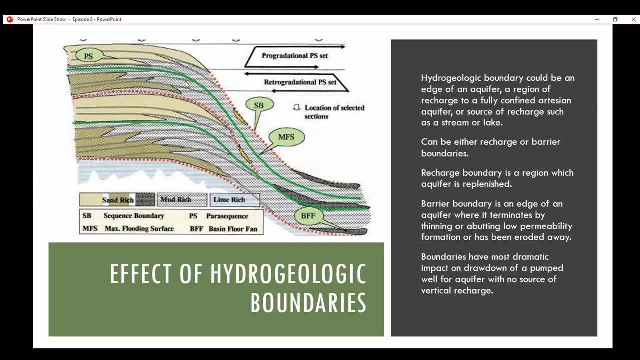 boundary to this potential aquifer right here, which is a sandstone and let's just say it's. it has a good hydraulic conductivity. so boundaries have the most dramatic impact on drawdown of a pumped well for aquifer with no source of vertical recharge. so basically, a clay is what it's talking. 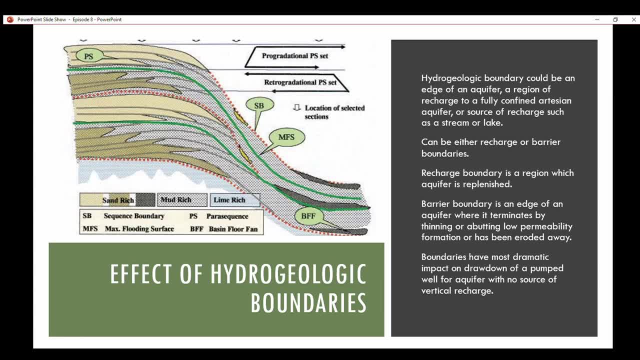 about there. but I have a lot of situations where I'll pump a well and it'll go dry after the first well volume. it won't even make it to the three. so in that case we just we sample, we wait until it reaches a certain point, a certain elevation, before we sample it. but yeah, so this is the. 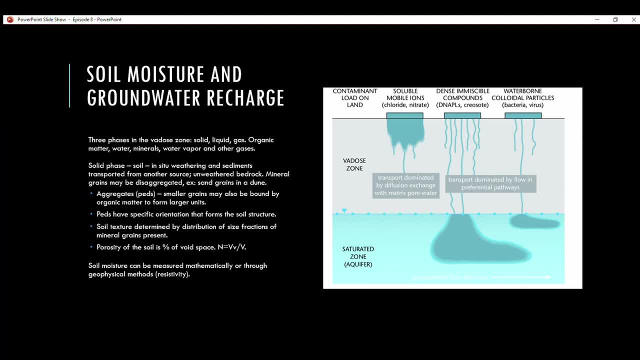 second one. the last one's going to be the second one is going to be the third one right here. so part of the episode: soil, moisture and groundwater recharge. so there's three phases. in the vado zone, or the unsaturated zone, there's a solid liquid and gas. you have organic matter, minerals, as your. 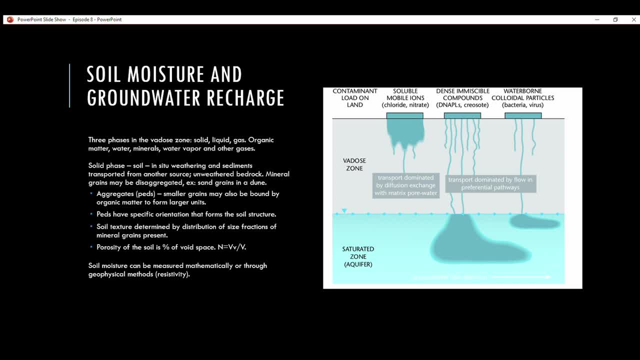 solids, and then you have water as your liquid, and then you have water vapor and other gases as your as your gases. so the solid phase, which is soil, is which can be created through in-situ weathering or from sediments transported from another source, or it can be created from unweathered bedrock. 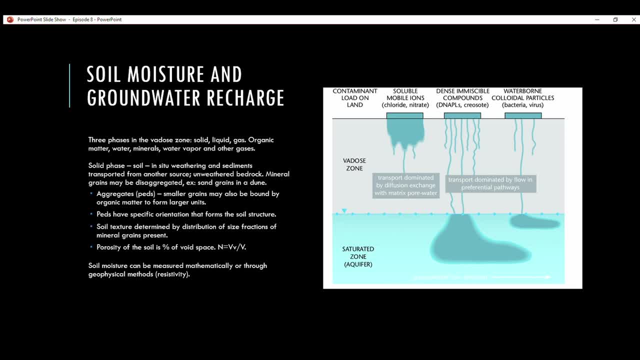 which is in this case in-situ weathering. mineral grains may be disaggregated, such as sand grains in a dune. aggregates or pads are smaller grains that may be bound by organic matter to form larger units, and pads or aggregates have specific orientations that form soil structures. 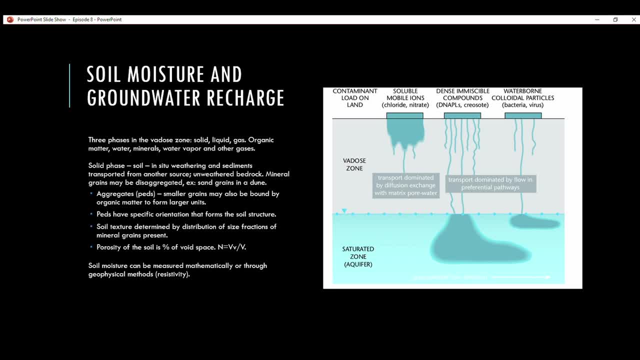 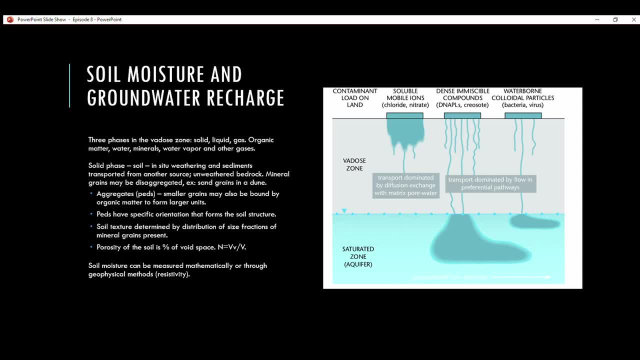 of mineral grains present and kind of review. porosity of the soils: percent of void space porosity equals the volume of the voids divided by the total volume of the of the material. so, and then soil moisture can be measured mathematically or through geophysical methods. 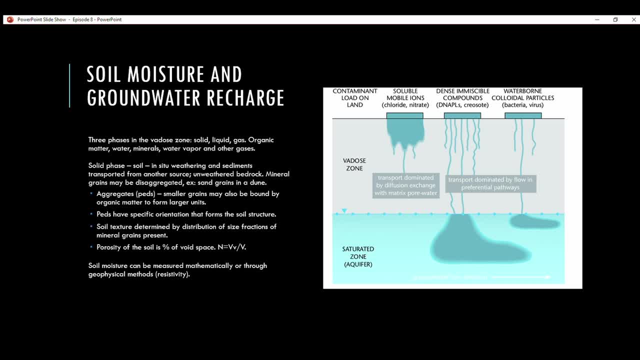 such as recidivity, and i i kind of like this picture. it kind of shows you know how pretty much unsaturated the uh, the uh, those zone ends. but you'll have uh leakage towards the? uh the saturated zone or the free addicts own. 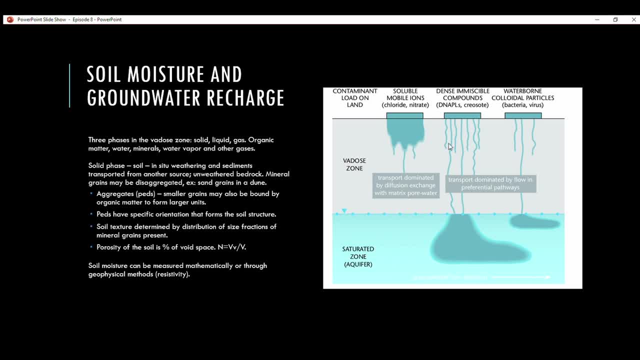 through fractures were, these are dead. this means dense- uh sorry for Dense non-aqueous petroleum liquids or product. We can just call it product, but I like this picture. I'm kind of showing, you know, the VEDO zone isn't completely saturated. It can have maybe some saturation near the top and then it'll dry out, or, you know, saturation right here in the capillary fringe. 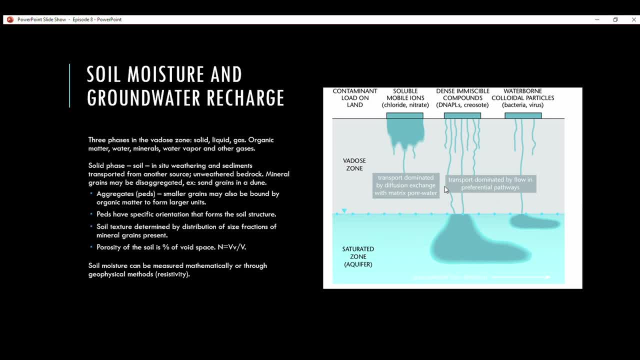 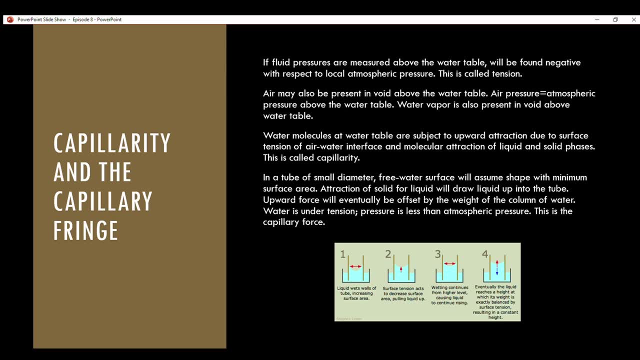 And speaking of capillary fringe, capillarity and the capillary fringe, if fluid pressures are measured above the water table, the pressures will be found to be negative with respect to the local atmospheric pressure, And this is called tension. Air may also be present in the void above the water table If the air pressure equals the atmospheric pressure above the water table. water vapor is also present in the void. 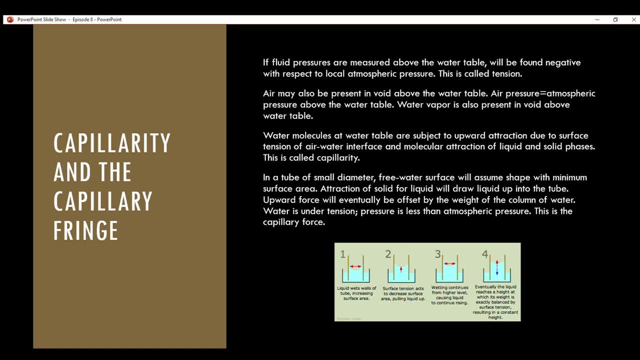 Water molecules at the water table are subject to upward attraction due to surface tension of the air-water interface and the molecular attraction of liquid and solid phases, and that's called capillarity. And in a tube of small diameter free water surface, it will assume sorry, free water. the free water surface in the tube will assume the shape of the capillarity. 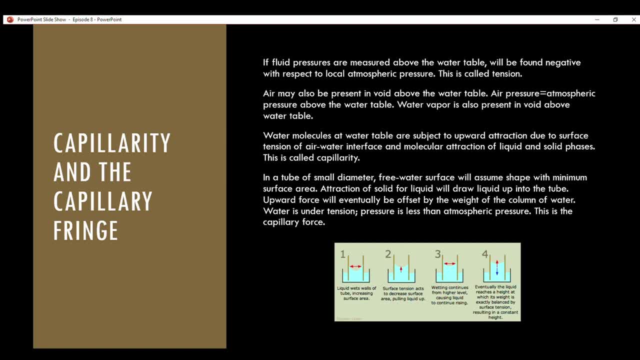 The capillarity is the shape with minimum surface area. The attraction of solid for liquid will draw liquid up into the tube. The upward force will eventually be offset by the weight of the column of water. Water is under tension. Pressure is less than atmospheric pressure. This is the capillary force. 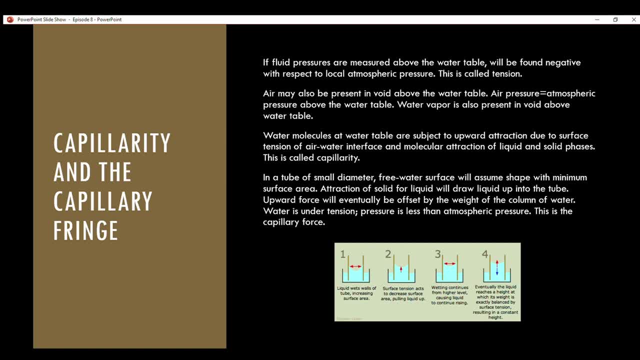 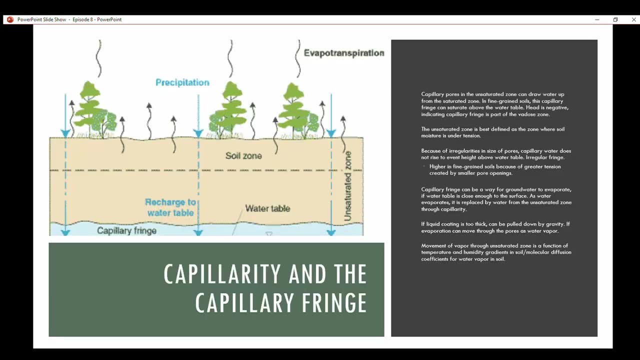 And this is a good little diagram to kind of give you a visual on how capillarity, the capillary force, exists. Okay, so the capillary pores in the unsaturated zone can draw water up from the saturated zone. In fine-grained soils this capillary fringe can saturate above the water table Head is negative, which indicates the capillary fringe is part of the vetos zone. 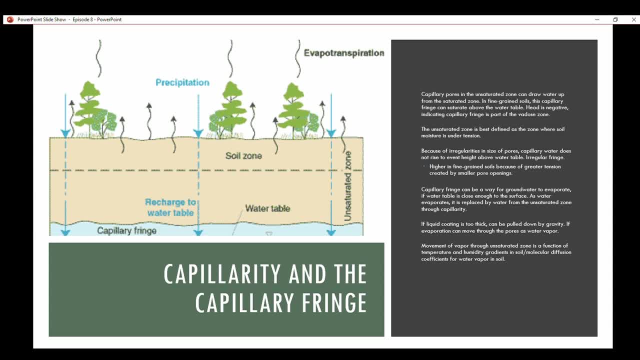 The unsaturated zone is best defined as the zone where soil moisture is under tension. Because of irregularities in size of pores, capillary water does not rise to even- even- that's supposed to be even- height above the water table. it creates this irregular shape above the water table. 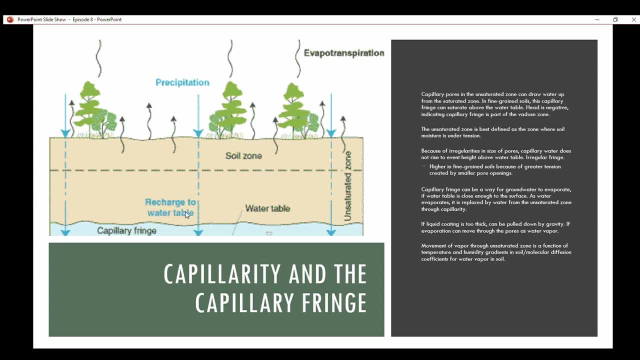 kind of hilly, looking higher, and fine-grained soils because of the greater tension created by smaller pore openings. and when you think fine-grained soils you think silts and clays. capillary fringe can be a way for the groundwater to evaporate if the water table is close enough to the surface, as 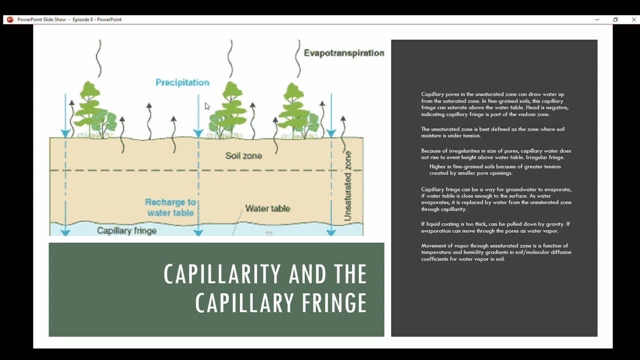 water evaporates, it's replaced by water from the unsaturated zone through capillarity. so you have water evaporating into the atmosphere. so water will in the capillary fringe, will go back down into the into the water table. if the liquid coating is too thick it can be pulled down by gravity, like 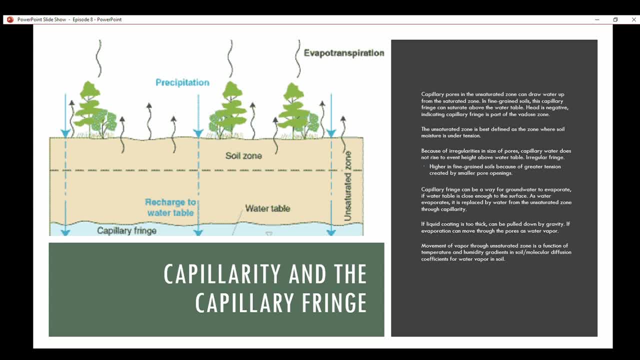 gravity. if the liquid coating is too thick, it can be pulled down by gravity if it's really saturated. basically, if evaporation can move through the pores as water vapor. I don't know why I put if, but yeah, evaporated water molecules can move through the pores as water vapor. movement of vapor through the 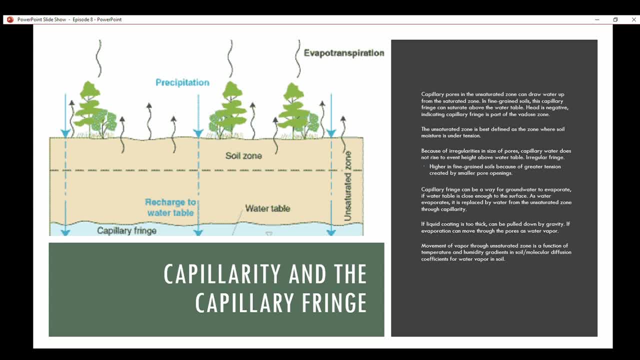 unsaturated zone is a function of the temperature and humidity gradients and soil molecular diffusion coefficients for water vapor and soil. so water vapor movement would probably not be very high in a place without humidity, such as an arid, desert southwest region of the United States, whereas in Louisiana this 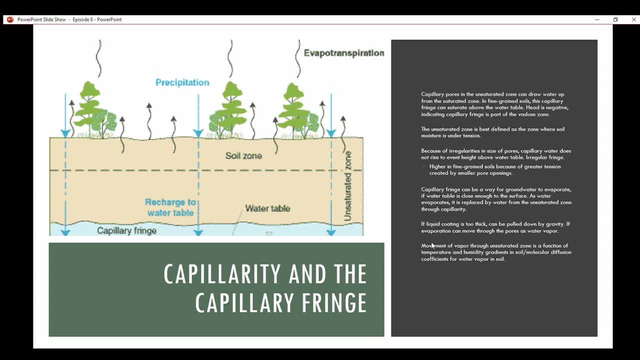 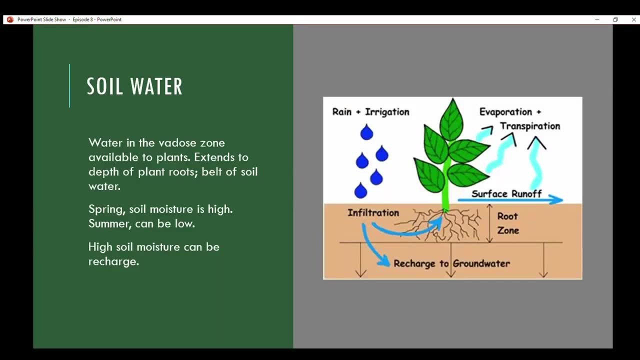 is probably, you know there's probably a lot of water vapor moving through the through pores. so soil water, water in the vetos zone that is available to plants. it extends to the depth of plant roots. you can also call it a belt of soil water, and water moves through this belt- spring soil. 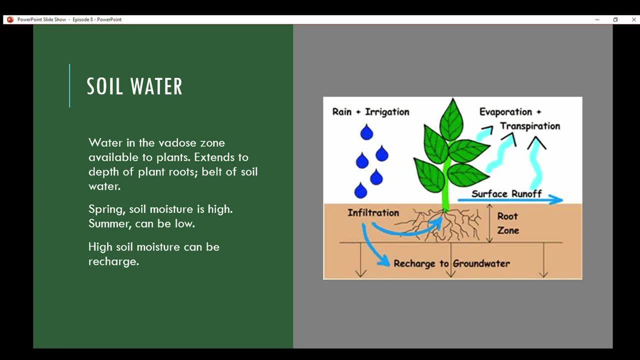 moisture is high due to snowmelt and, in some cases, high precipitation, and then in the summer it can be low certain places. you know you have your monsoon season, so maybe so my moisture is high during certain portions of the summer and then when you're dealing with high soil moisture it can be used for a lot of.